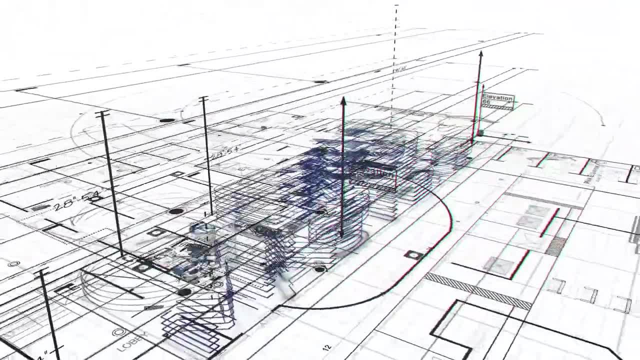 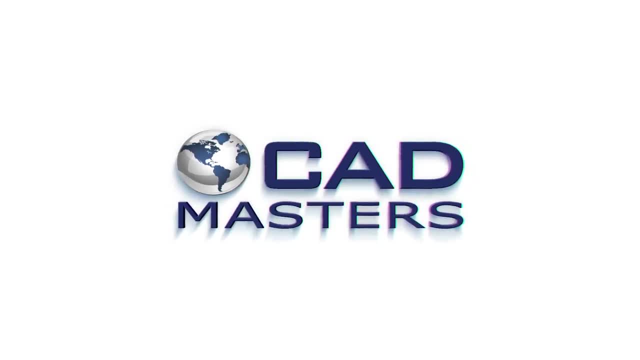 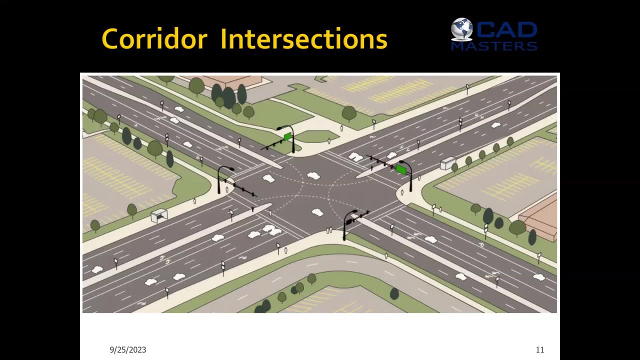 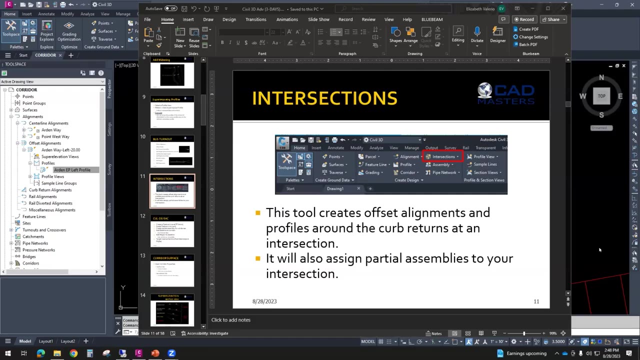 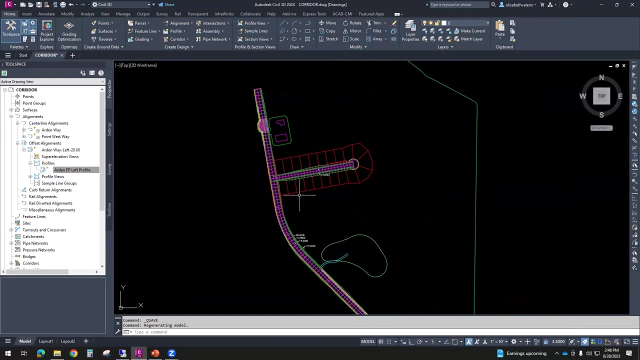 In this video you'll be watching an excerpt from our Civil 3D Advanced class. The topic being covered is corridor intersections. So our topic that we're going to cover right now is intersections. If we look at this project, we have Arden going north to south and we have Point West going east. 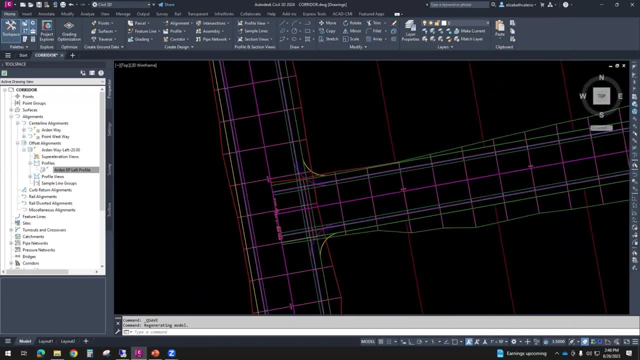 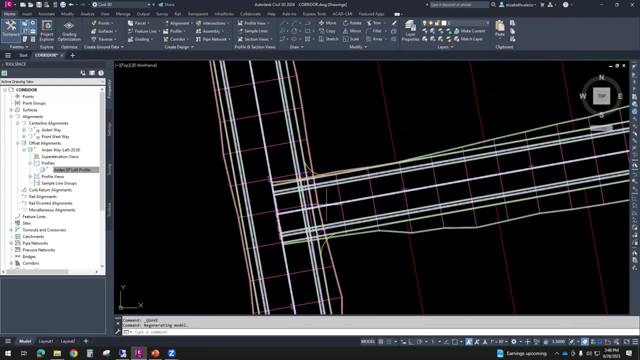 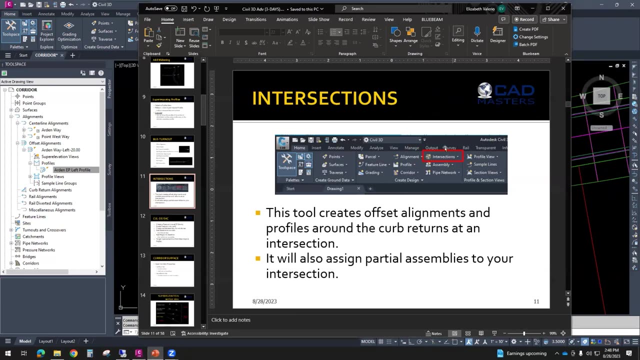 to west And right here is where they overlap, but it's not a nice, clean intersection. So what we're going to do is first open this up, remove the pieces of corridor that are in the intersection and then we'll go into this slide and talk about using the intersection button and how that. 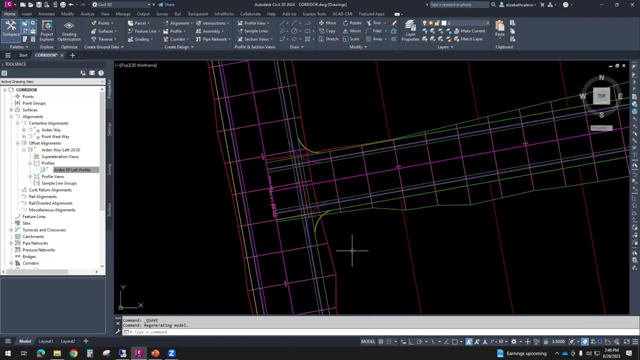 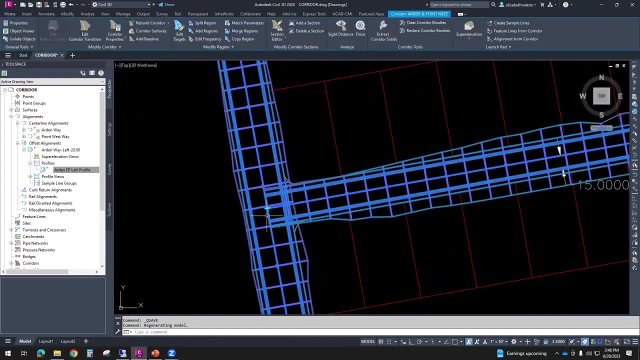 can help us clean it up. Okay, so first, looking at what we already have, let's click on the corridor And you'll see there's a diamond grip at the end of Point West. Click on that diamond grip and just pull it out of the intersection. Let's give extra space. We'll just pull it all the way to here. 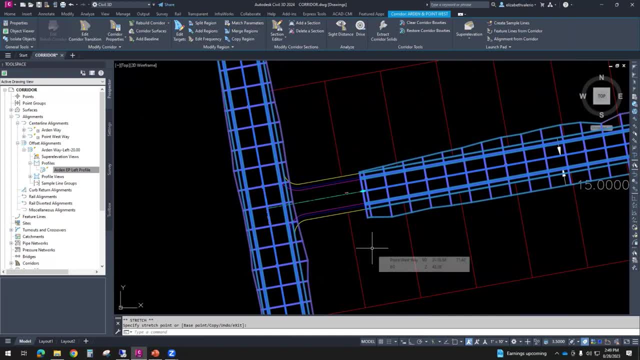 Later on, if we need to pull it back, we can always pull it back. Then for Arden, we need to split this. Right now it's one foot, So we're going to use the split region. So when I select the corridor up in the ribbon, we have split region. 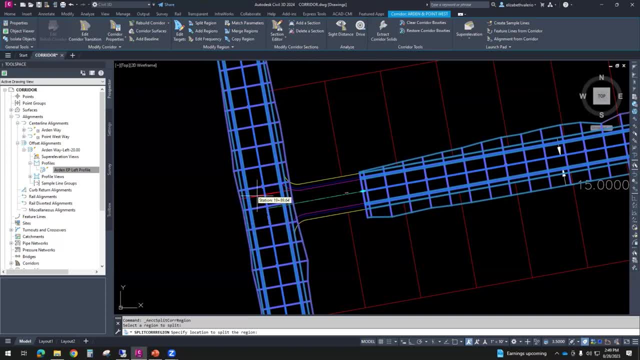 And we've used this before. We select the region And we get that red line, And this time it doesn't have to be very specific. I just want to get plenty of space. I'm going to click up here to split before the intersection. 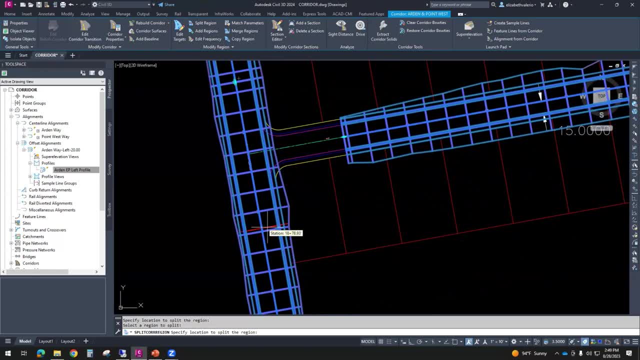 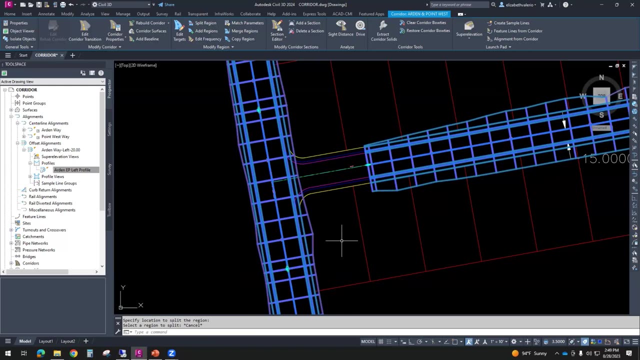 And then I'll click in this region down here. use the red line again, Click somewhere after that intersection So you should see diamond grips above and below the intersection. Once it's split we're going to delete this region. So with the corridor selected up in the ribbon under modify region, we have delete region. 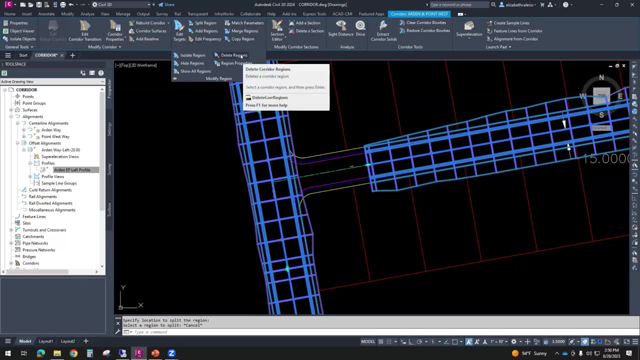 So with the corridor selected up in the ribbon under modify region, we have delete region. So with the corridor selected up in the ribbon under modify region, we have delete region. And then you're going to have to click twice, Click once to select the region. 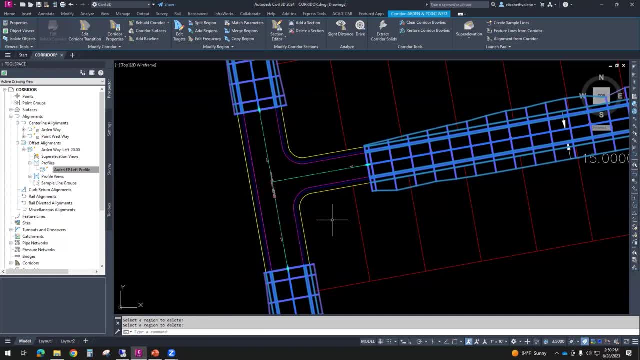 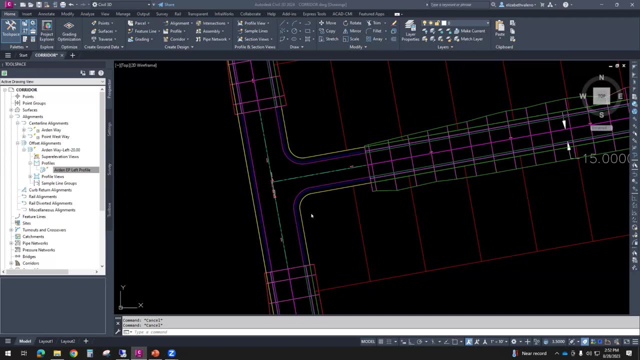 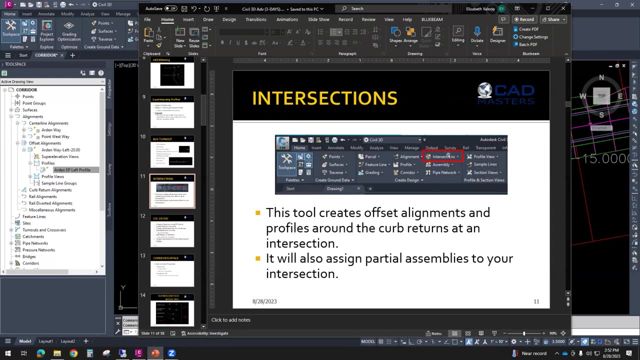 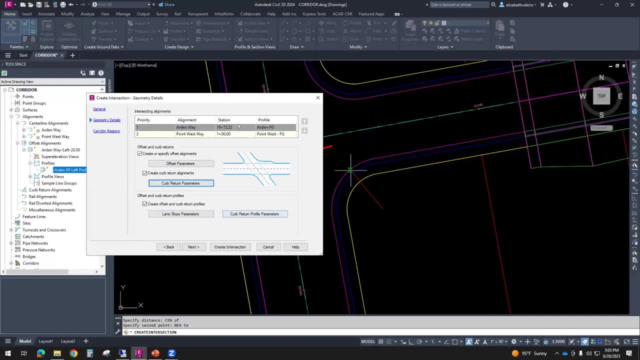 So in the home tab of the ribbon in the create design panel we have the intersections button. So in the home tab of the ribbon in the create design panel we have the intersections button. Next we need offset profiles. So we need to give it some slope information. 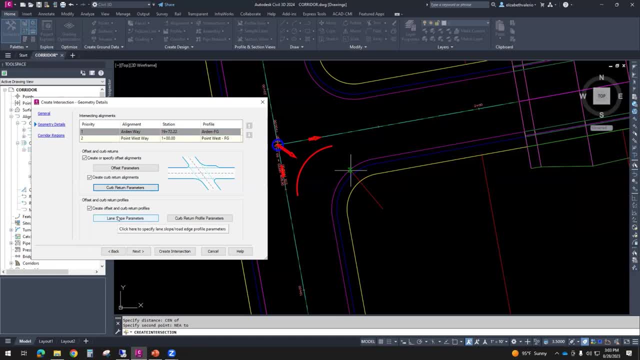 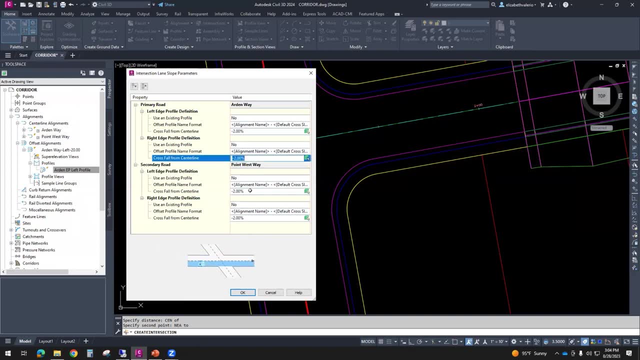 Let's click lane slope parameters In here. it looks good. We have a 2% cross slope for all the roads right, Left lane, right lane, Arden Point, West- All of them have the 2% cross slope. 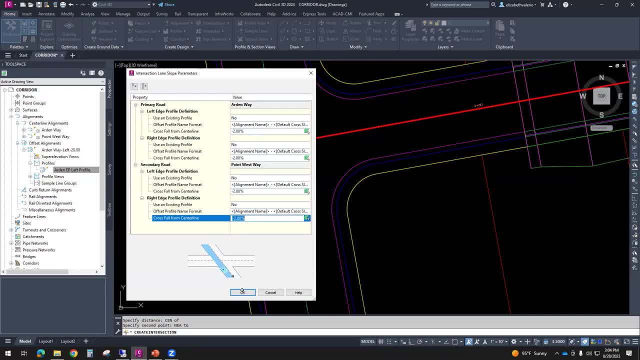 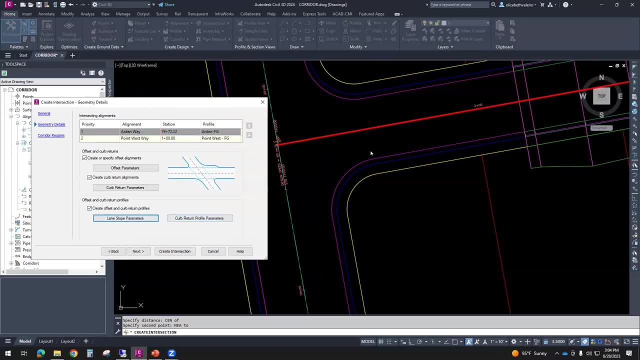 So that looks good. Okay, Great, Katina, Perfect, Perfect. And then here curve return profile parameters. So this first button was for the cross slope here. The second button is for the cross slope here. Let's see what other parameters we need to look at. 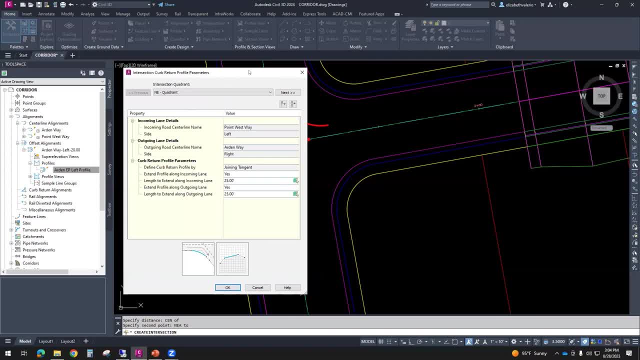 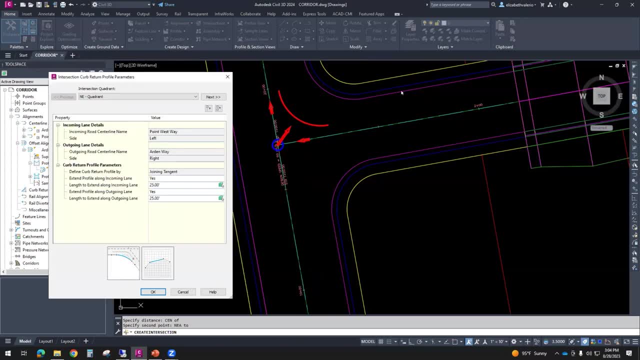 Actually it's not even about slope, but it is about going around that curve. So it's going to follow the 2% cross slope all the way down here And then it has to just kind of transition around that curve and then end up well, I. 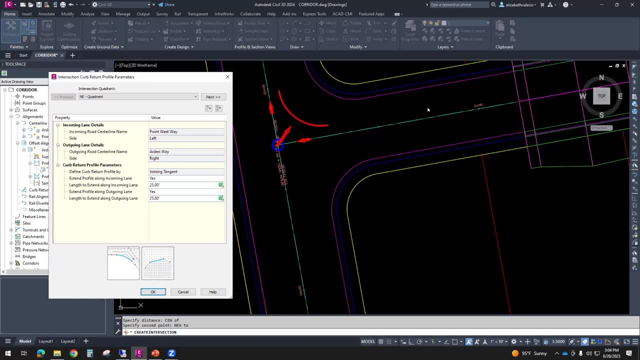 guess, if I show it this way, it's better. It's going to come follow the 2% cross slope on this street all the way to here And then it needs to transition around the curve to whatever this ends up being, with a 2% cross slope from that street, right. 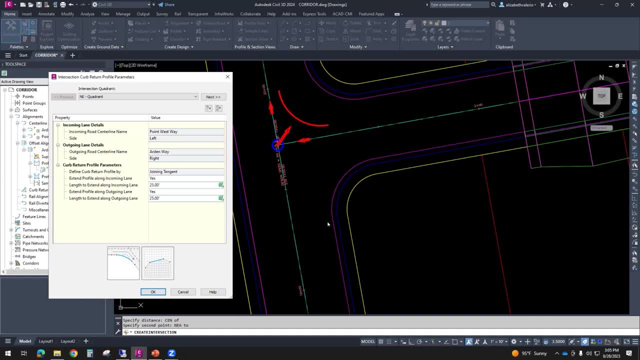 So going around the curve is just actually a transition. However, we can tell it, rather than going Following the profile all the way to this end point, we can stop a little bit short and kind of ease into this transition, right? So rather than going all the way to the end point, we stop a little bit short and go ease. 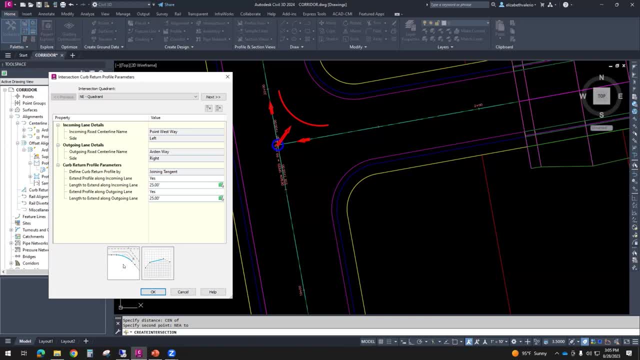 into this transition around the curve. So this is a plan view going around the curve And this is a profile view. what it would look like? a slope, a constant slope going around that curve. The transition Is A little bit here and a little bit here in plan view, a little bit here, a little bit. 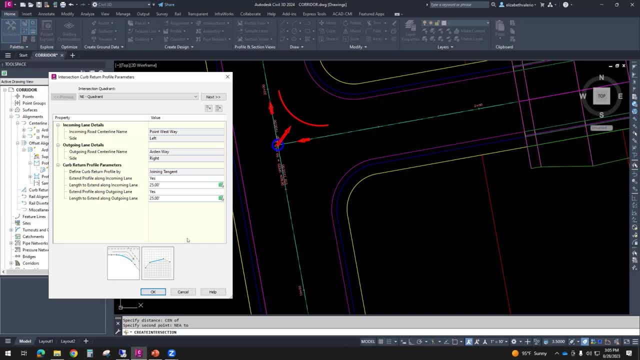 here in profile view. So it's asking us: do you want to have a transition? How long should that transition be? So here we'll say: yes, we want a 20 foot- 25 foot transition going into the curve, And then we want another 25 foot transition going out of the curve. 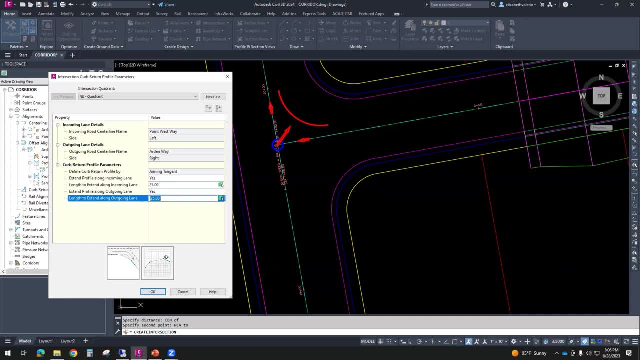 So it won't be so dramatic how it looks in this profile where it's like straight up, straight down. It'll ease it into that that curve more. So we're talking about profile right. We're trying to try to have a more gradual slope as it goes around this curve. 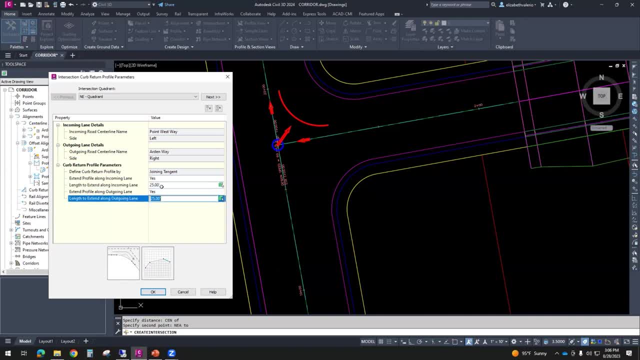 Does that make sense? You could change these numbers if you want the transition larger or smaller, but I'll stick with those defaults. Right? There are two quadrants, the north east quadrant and the south east quadrant, so make sure you check both of them. 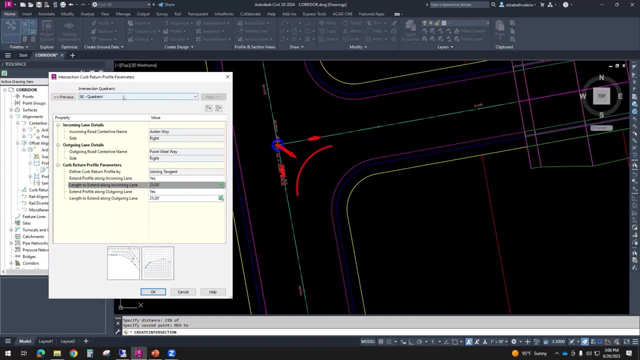 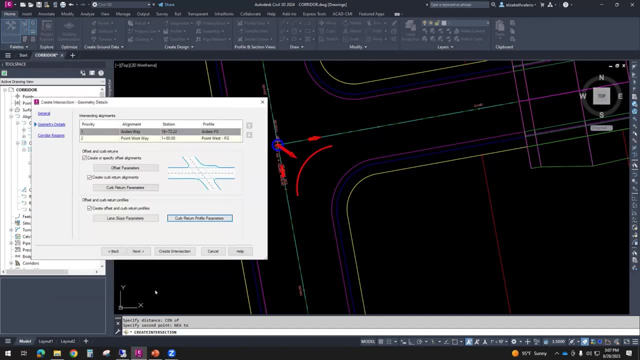 We're going to stick to the 25 foot transition. Click OK. All right, So we're done with this window. We have set up the alignment and profile parameters. We'll click next. So this is where it gets more complicated. See, we make this bigger. 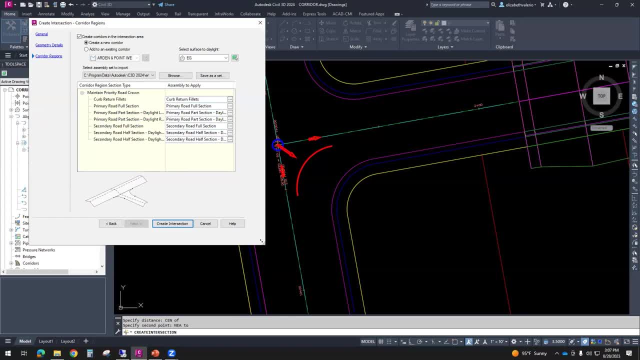 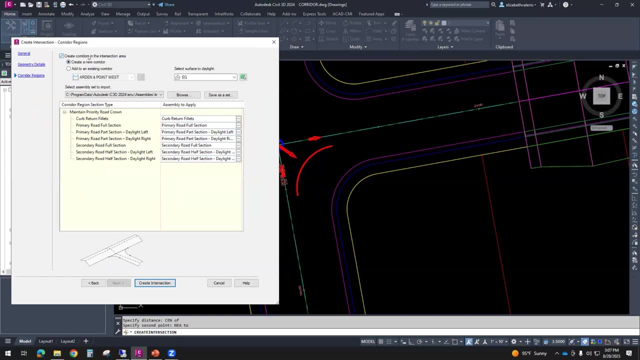 We're going to add a new border. We're going to add a new border to our existing corridor. We're going to add a new border to our existing corridor. So up at the top, there's an option here: Create corridor in the intersection area. 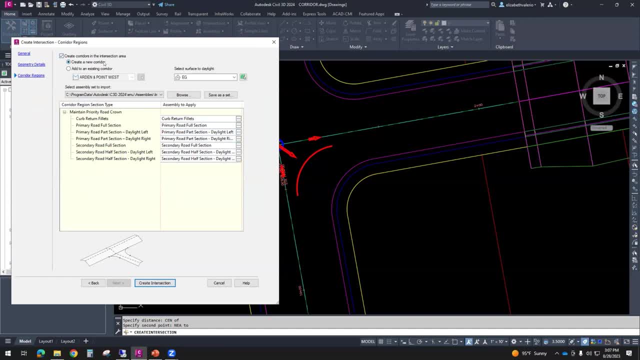 Yes, we want that checked. Create a new corridor or add to an existing corridor, So I don't want this to be a separate corridor. I want to add the intersection to my existing corridor. My existing corridor is Arden and Point West. 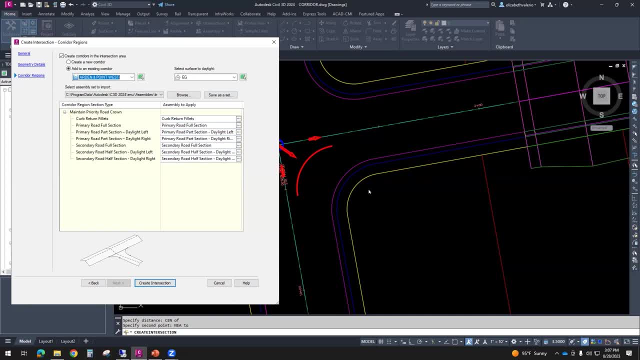 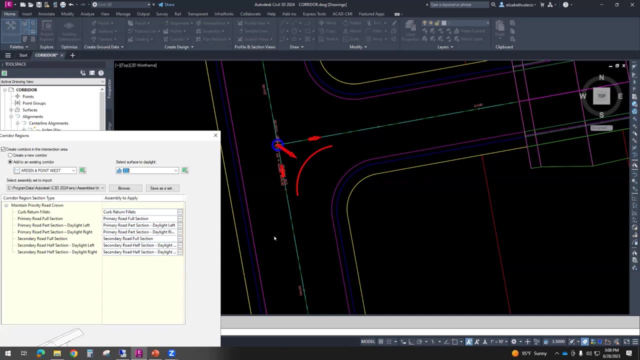 It will have some daylighting around the edge around here. So if we daylight, we want it to daylight to the EG surface. So that's the target, Okay. and then now these are the assemblies So I mentioned earlier. it's going to use like one assembly that goes straight. 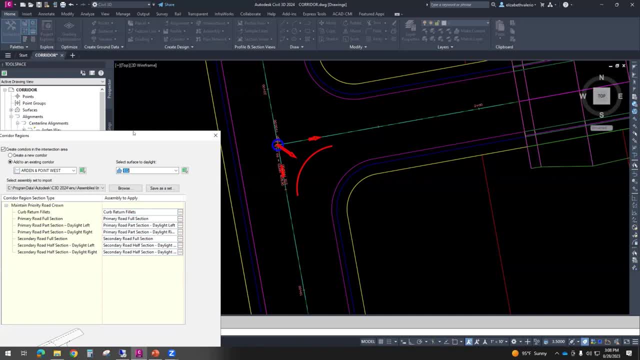 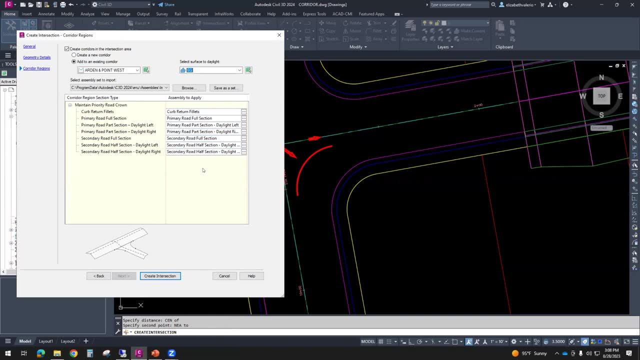 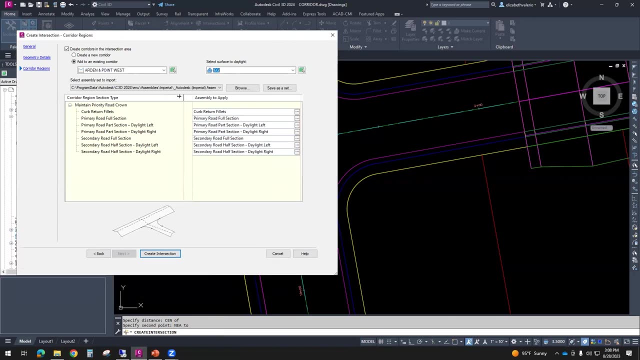 Another assembly that comes around the curve comes around the curve right, And so these are the default assemblies that it will be assigning. Let's see if there's anything that we can trade out right now, because, I mentioned, the default assemblies don't necessarily follow our design criteria. 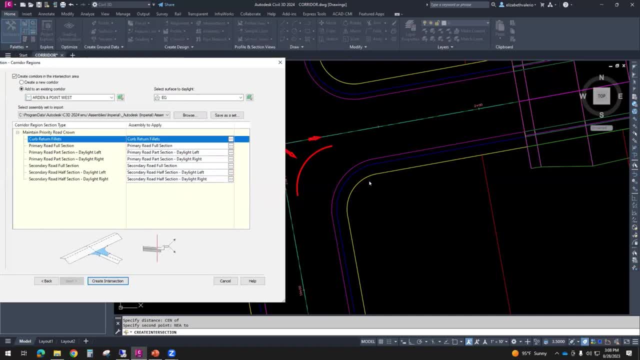 So curb return. fillet is something that is probably going to use around this curve. Primary road, full section. So primary road is Arden, Full section is our original assembly, So let's switch this out right now. Click the dots Or the button with the dots. 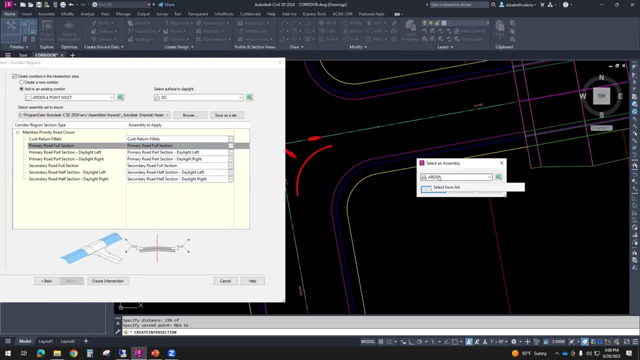 Arden is the primary road And this is the full section assembly. Click. okay, Make sense. Question: Primary road part section daylight left. We're not sure about that Primary road part section daylight right. Not sure about that Secondary road full section. 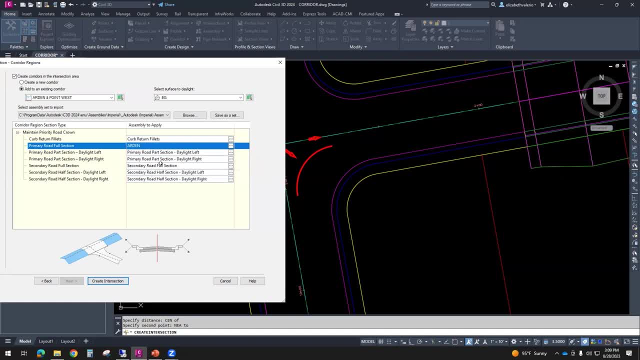 So secondary road is Point West And we do have the full assembly, the full section. So if I click the button with the dots I can switch this one to Point West. Secondary road- half section- daylight left. Secondary road- half section- daylight right. 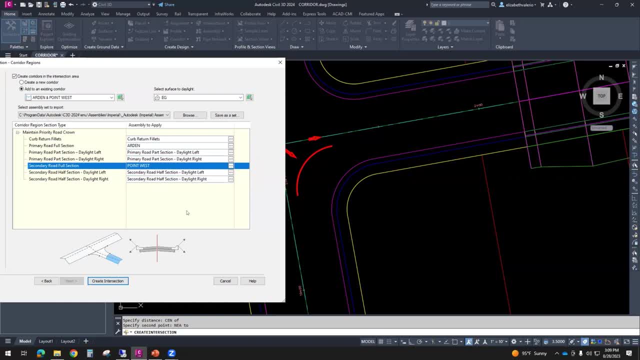 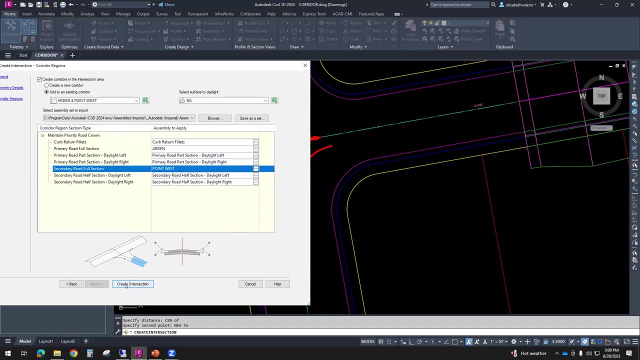 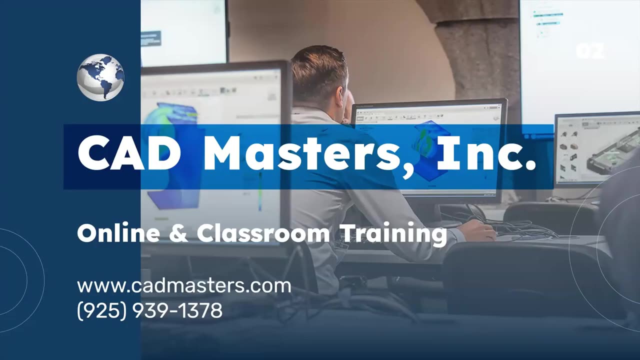 So these other ones, we're not quite sure what they are yet, So we're going to wait on those. Let's click create intersection And it's going to think for a little bit. Add Masters offers online and classroom training for a variety of Autodesk software. 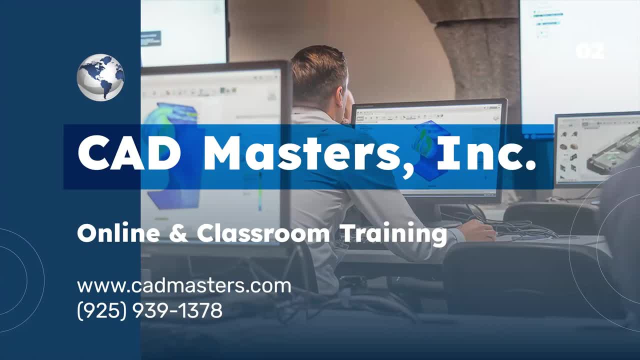 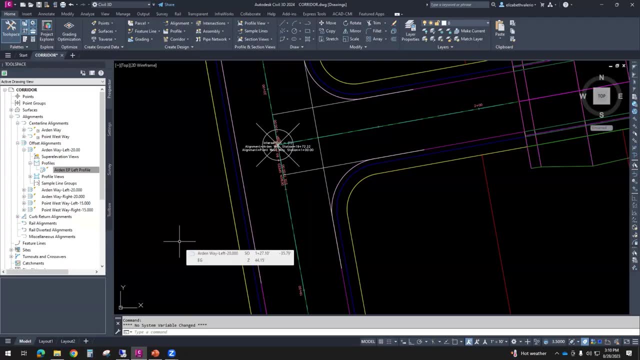 For more information, go to wwwcadmasterscom or give us a call at 925-939-1378.. So, if your drawing is like mine, what you're looking at are the new offset and a lot of Offset alignments. These are the offset alignments. 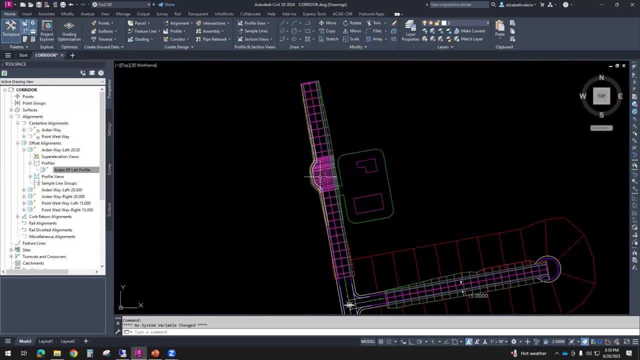 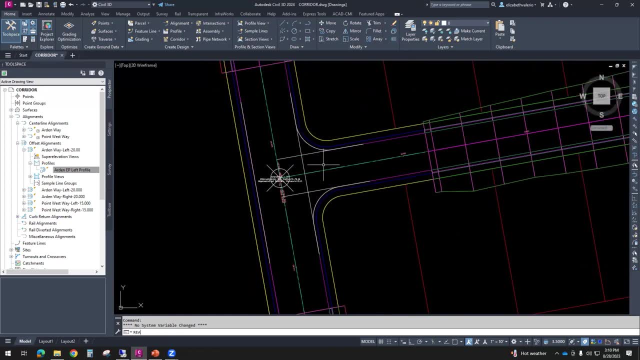 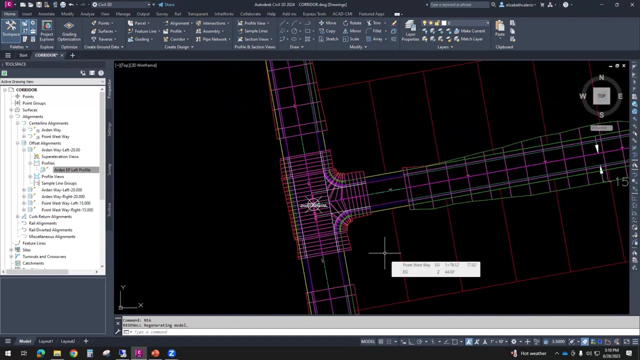 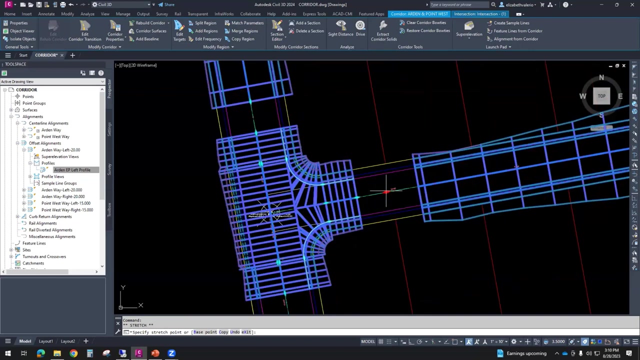 Remember when we worked on it up here just showed a white line. These are those white lines, those offset alignments. If I regenerate re a enter now I can see the corridor intersection. Okay, so you can click on the corridor and you can put the diamond grip to slide the corridor, and for everyone. 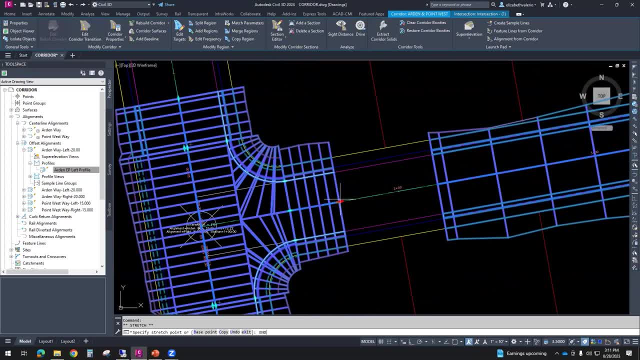 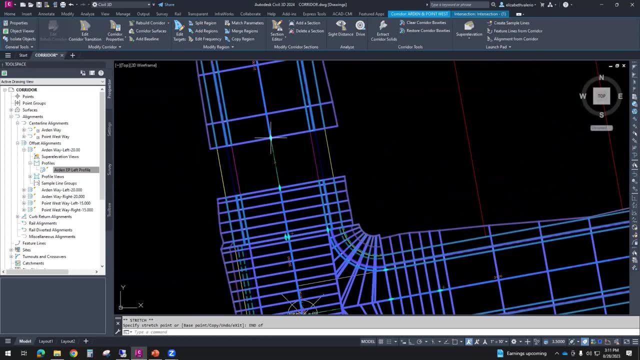 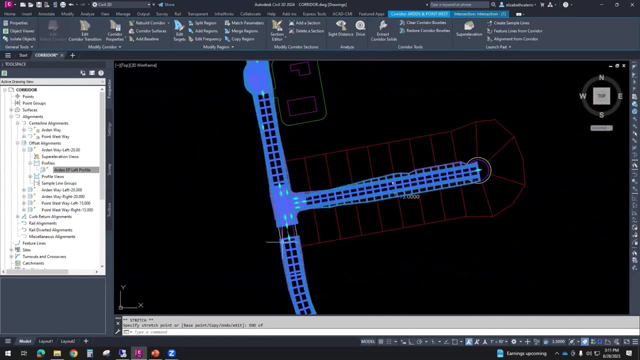 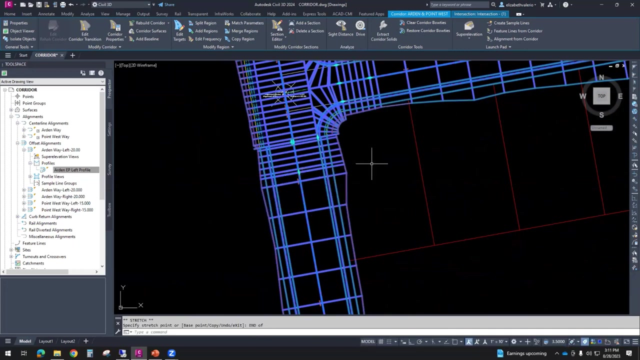 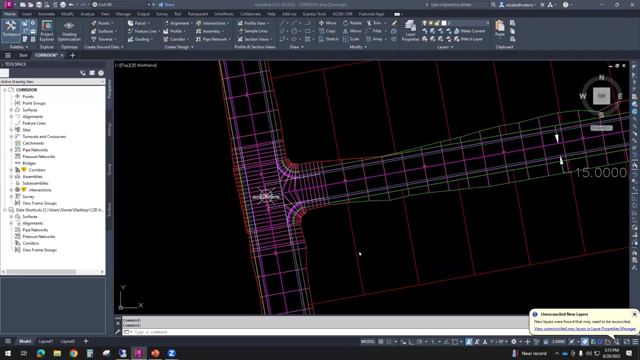 We're going to be sliding them so that they snap to the end of the intersection piece, So it should match up When you slide them in. So what I want to show you here is we have replaced, or let me show you the properties. 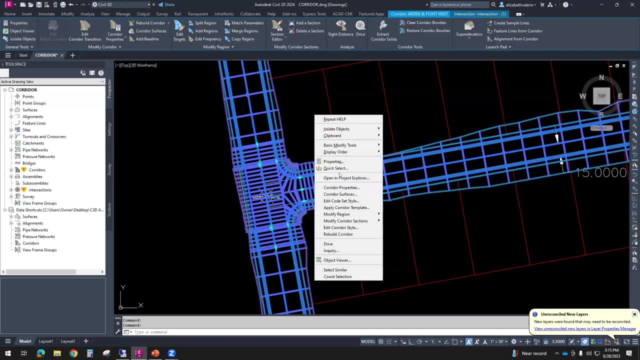 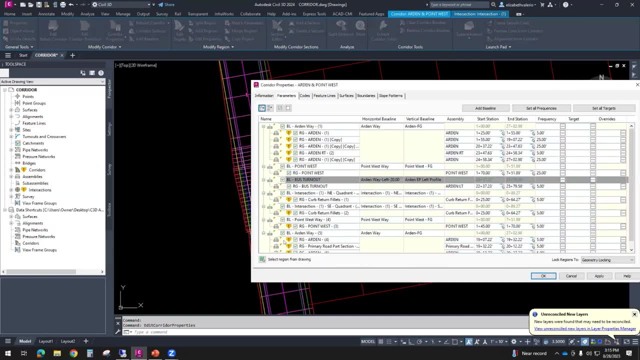 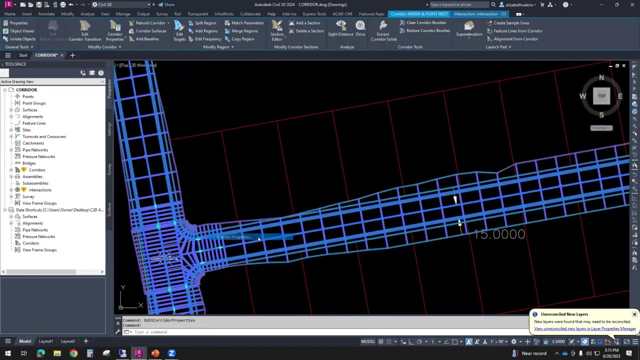 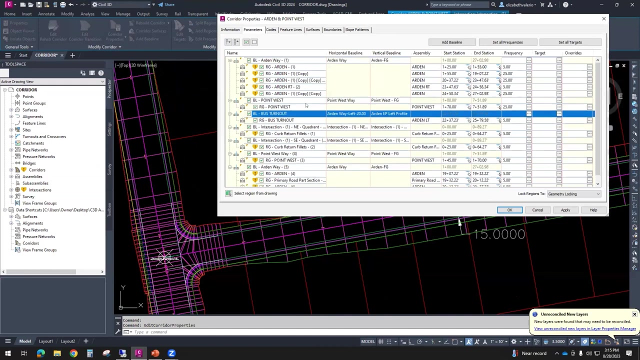 So if I grab the corridor, right click and go to corridor properties, It's hard to show you my screen and the corridor at the same time. There you go. Okay, There's a ton of stuff in corridor properties now. We had started with Arden baseline, Point West baseline, and then we added the bus turnout baseline. 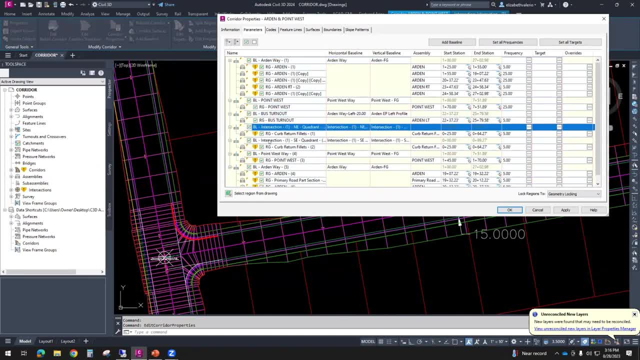 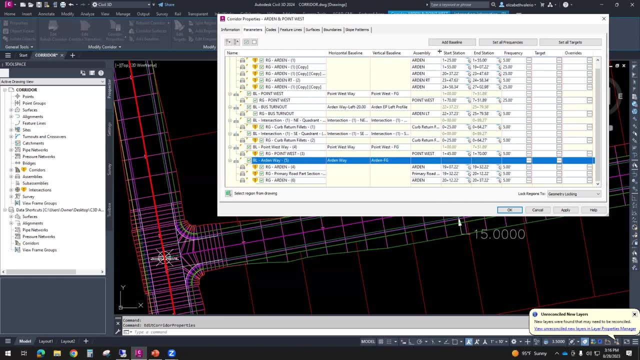 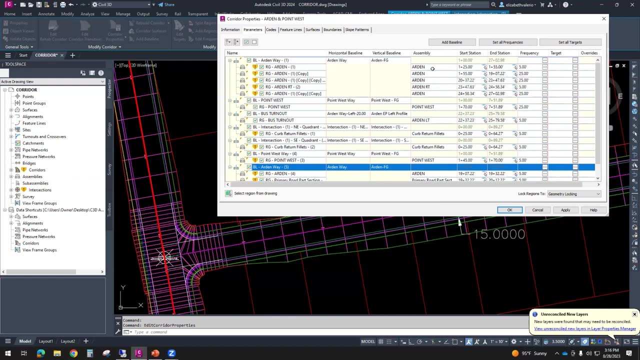 Now that we've used this intersection tool, We have a bunch of intersection baselines that were added automatically And if we look at the assembly column We can tell which assemblies are the ones we created and which ones are the ones Coming from the intersection. 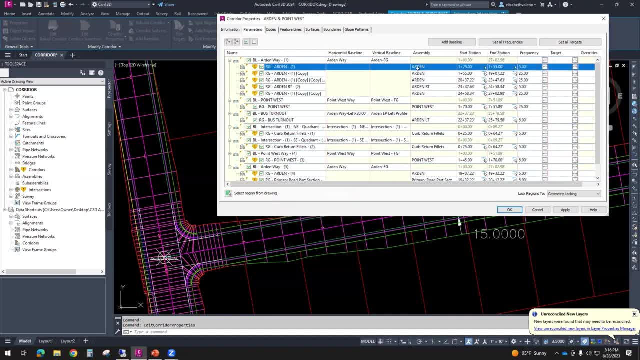 So Arden shouldn't click on it. Arden, Arden right, Point West, Arden left- those obviously we created. then we have these special ones: Curve return, fillet, curve return, fillet. Point West is something that we created and we has switched out in that window, in the intersection window, that we were working with Arden and Arden. 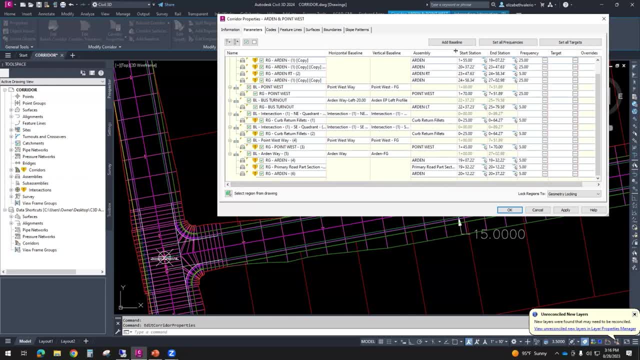 Those are ones that we created, that we have switched out in that Section window where these are being used. this Point West and these Arden ones are here. So there's the main road and there's the transition using the Arden cross section, Here's the main road and here's the transition using the Point West cross section, and then same thing down here right. 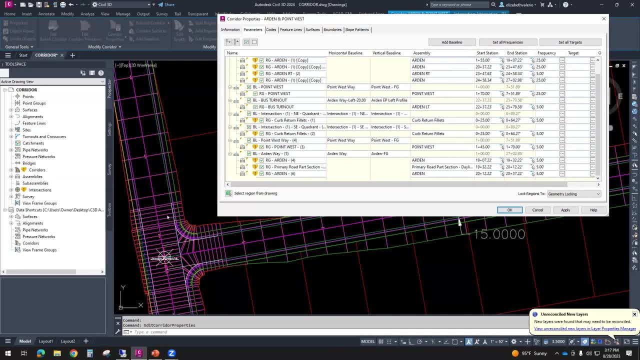 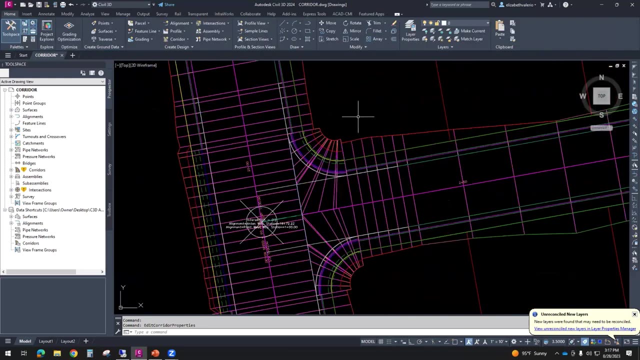 There's the main road and then the transition. So the transitions have already been set to the correct assemblies and they should transition nice And smoothly. shouldn't have any issues. But if we look closer, let me just cancel for a minute. You look closer. 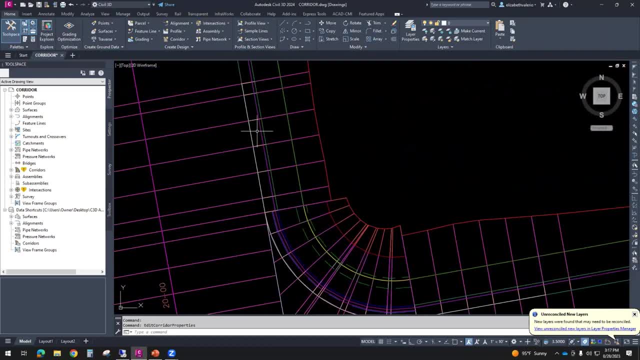 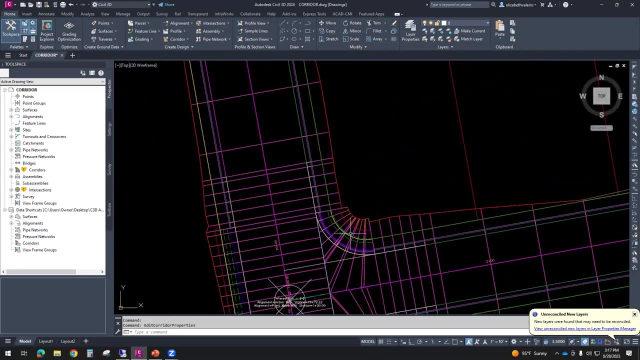 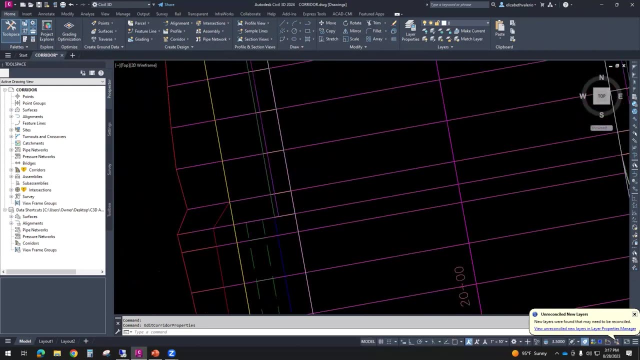 This curb return area. It does not line up right there. All these lines are off And that's because it's using its own default assembly. If you look at this area here, this is also kind of weird. We don't know what's going on here. 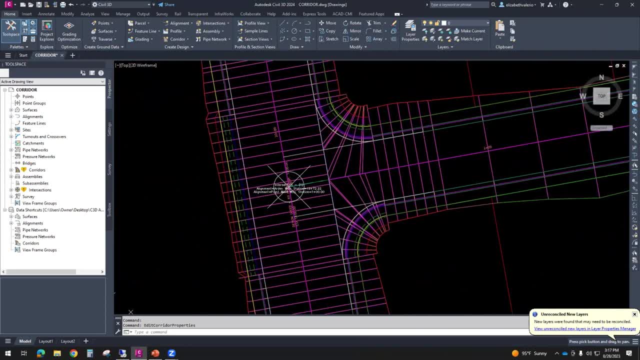 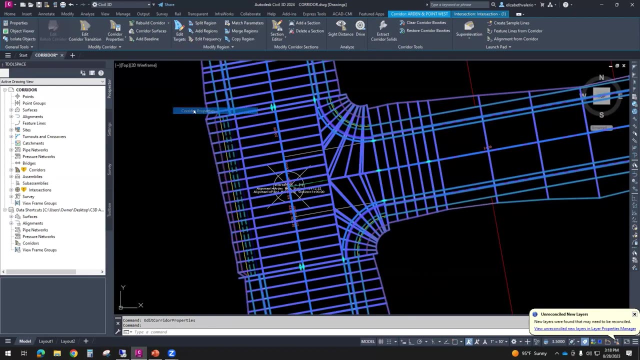 It doesn't match up with our Design. So there's three areas- One, two, three- where it has some funky line work coming from these additional assemblies that just showed up. If I look at corridor properties, I can take note. 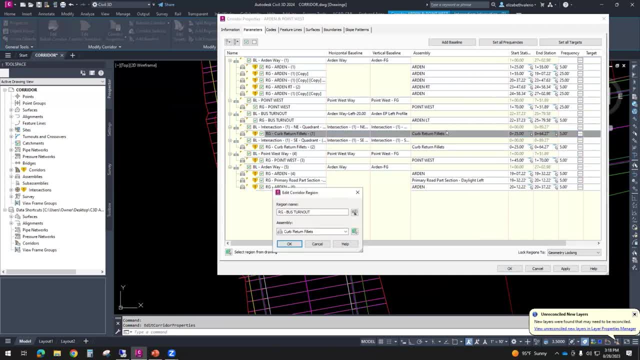 What these funny ones are right. So there's one called curb return fillet. Every time I click it opens. So there's only put this in the chat, that way We can keep track. So we have one called curb return fillet. 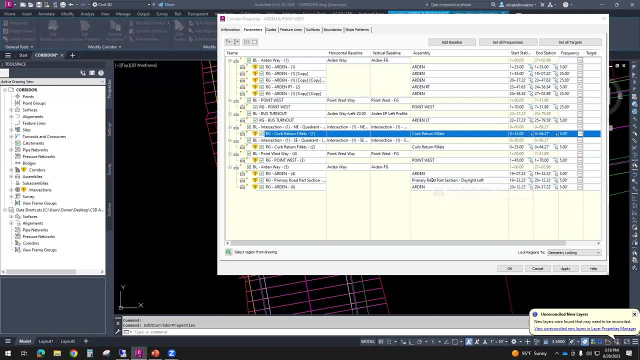 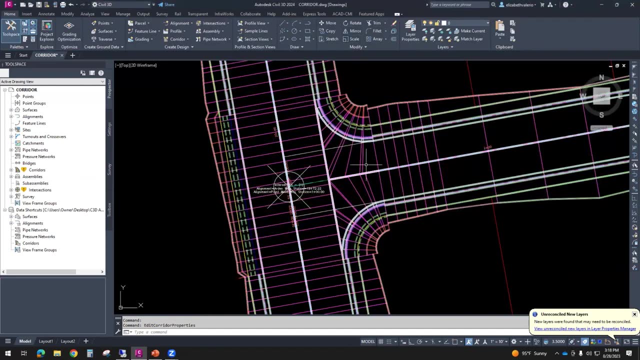 We have it used twice. And then we have one called primary road part section daylight left- put that in the chat And that one is used one time, So just taking a note right now. So these two look like curb return fillet and that one looks like primary road part section daylight left. 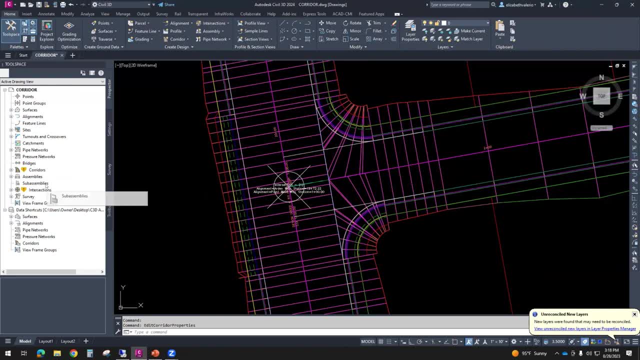 Where are these assemblies? You can see them two places. One is in tool space under assemblies- Again, you can tell the ones that I created and the ones that just randomly showed up- And then another place you can see them is in the actual model. 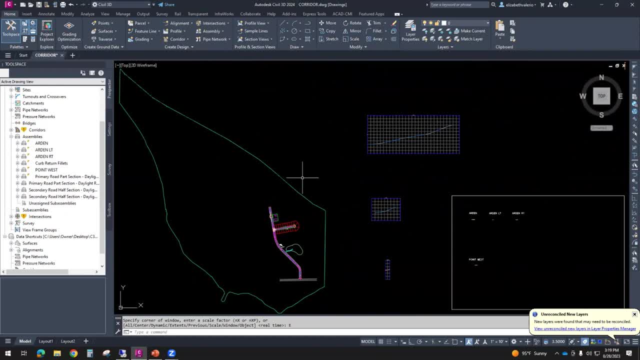 If you zoom extents, They are typically in the upper right corner. So zoom in here. These are the random Assemblies that it generated. So let's zoom in, Let's see which ones we need to actually deal with. So this first one. 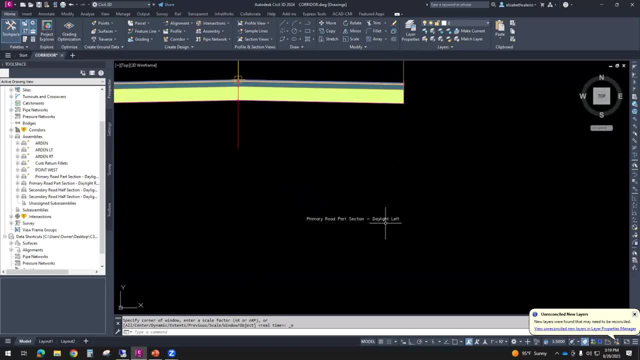 I don't need This one. Primary road part section, daylight left. I do need this one, So I'm going to put a rectangle around it. So that's one. I have to deal with This one. Second areas: No, No. 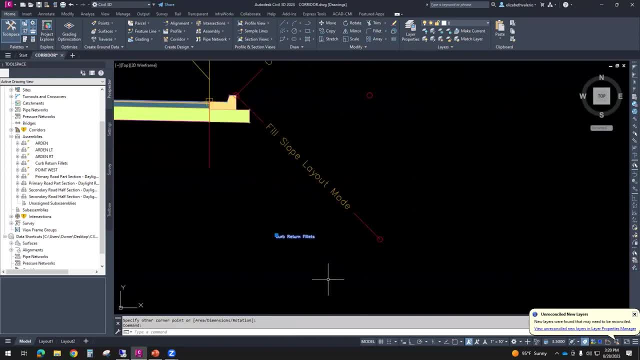 Yes, This is another one I need to deal with. Right Rectangle around that. So the reason why I know it's these two is because in my chat I wrote down what we actually have in our corridor Right, And so what I'm going to do now is kind of figure out. 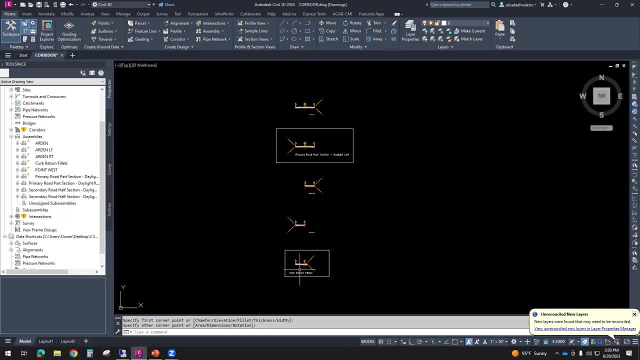 Why? Why pick this? and how it's different from what I need in my design. Let's start with this one: curb, return, fillet. Actually, let's do this. Grab the whole thing, Move it. Just use the move command, Move it into where our other assemblies are. 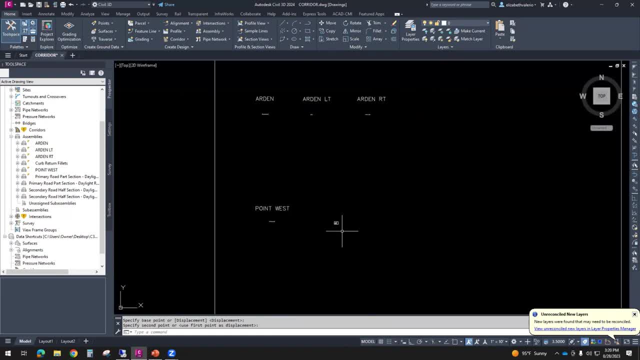 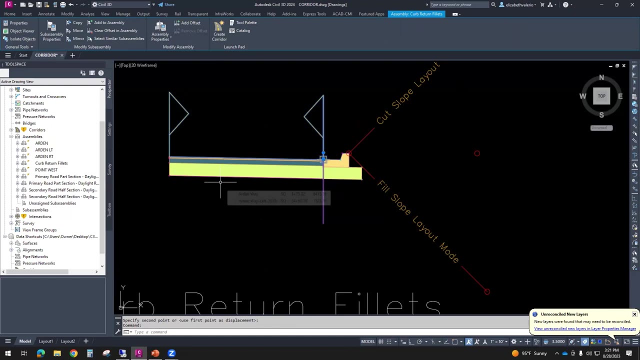 I'll just put it right here And then I'll zoom into it: Curb, return, fillet. It has The assembly line at the edge of pavement, It has a lane on the left And it has curve and gutter on the right. 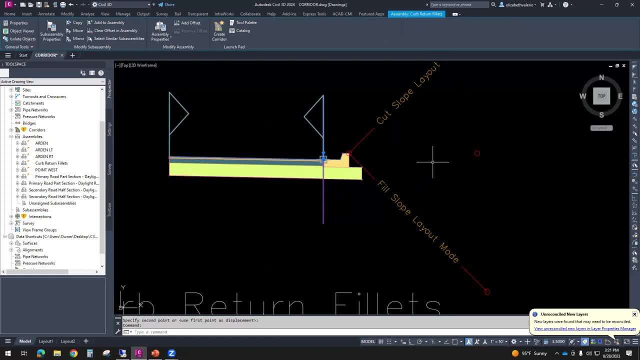 So what's missing is it's missing the sidewalk Before the daylight. it does have this daylight here, but it's missing the sidewalk Right. Do I have an assembly that looks similar to this? not that one, Not that one. This one is pretty similar. It's missing the lane. 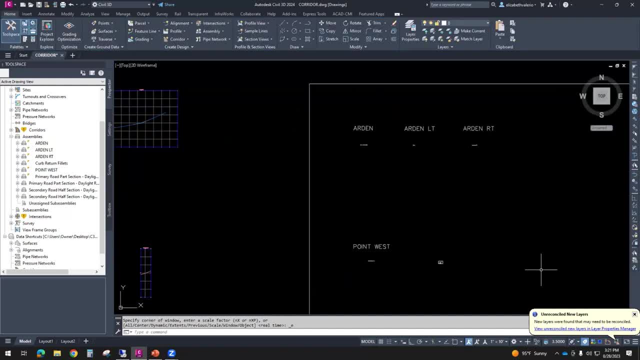 Not that one. So since there's none of them are exactly the correct assembly, let's just grab the Point West assembly. I'm going to grab it, copy it, put it right next to this one, But I'm going to give it a new name. So this one was called Curb Return Fillet. 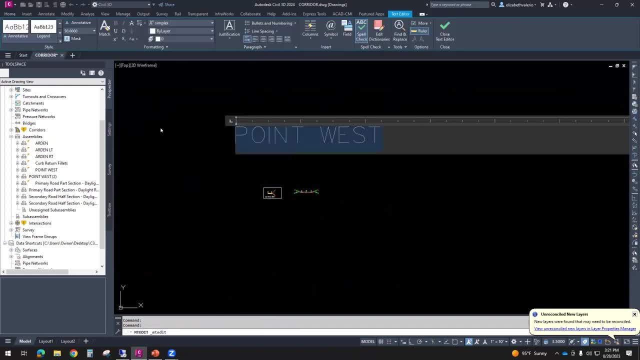 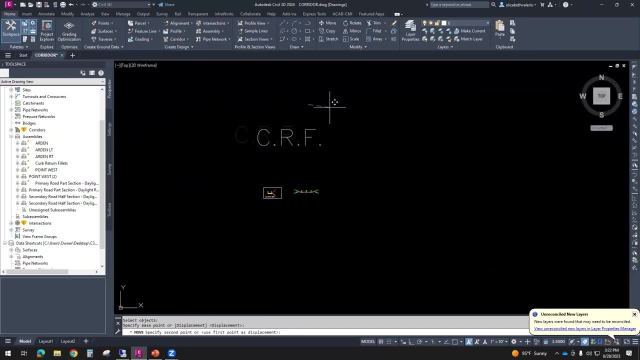 I'm going to call mine CRF Curb Return Fillet, And I want to make sure we're all caught up. but let me just give you one more step. So I copied this over, I copied Point West over, I changed the text. 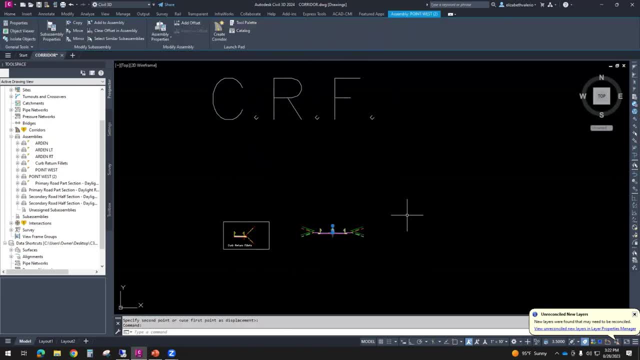 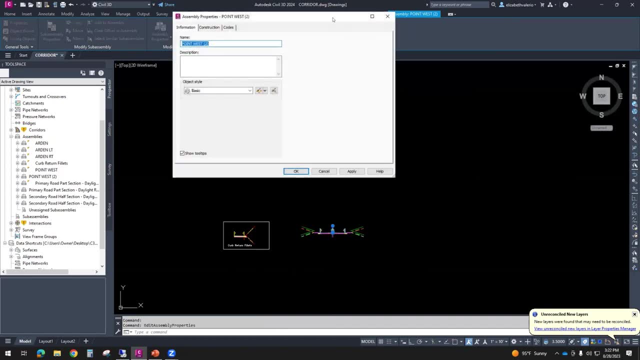 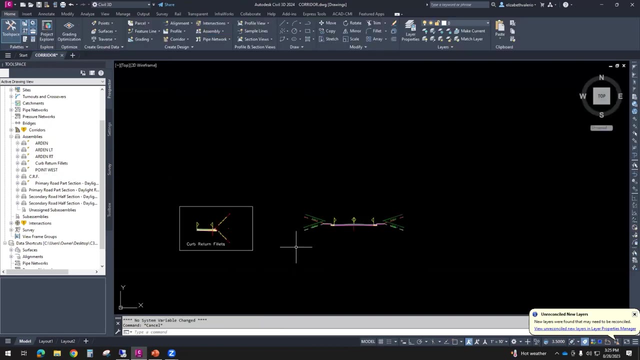 And I'm also going to go into the properties of the copied section Here: Assembly Properties. Since I copied it, it's called Point West 2.. I want this to be called CRF Curb Return Fillet. All right, So I have copied it. I've renamed it. 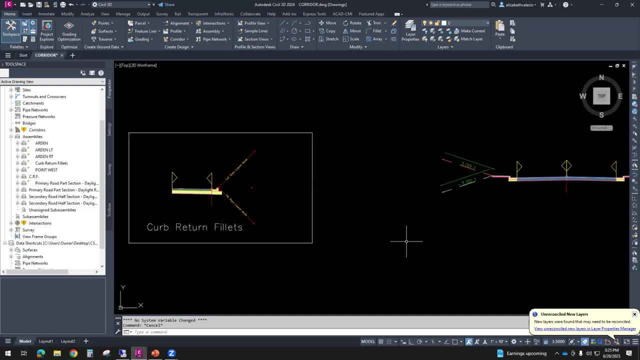 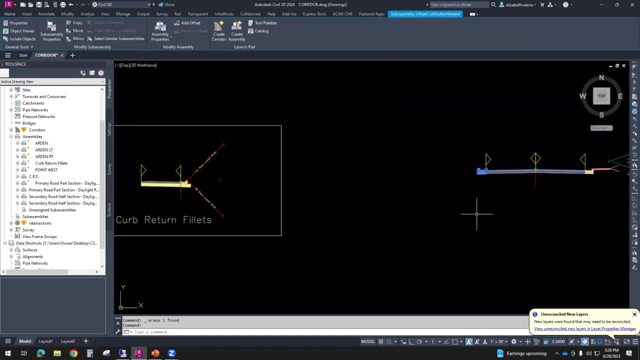 And I have the Curb Return Fillet right next to it, So I need to make my copy look like the Curb Return Fillet version. So, left side, I can delete the data. I'm going to go to Daylight. delete the Sidewalk, delete the Curb and Gutter. 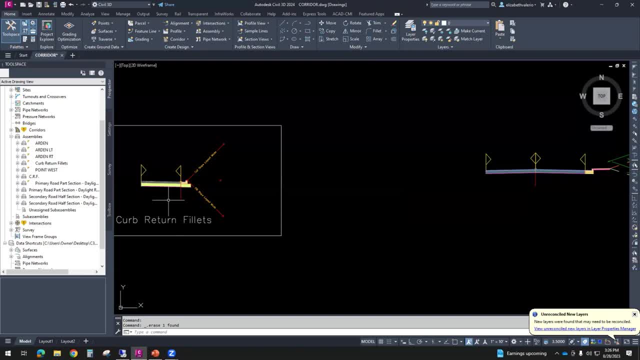 Notice how there's a lane on the left side of this assembly line, So don't delete the lane On the right side. I don't have a lane, so I'm going to delete the right lane. However, the slope is going the wrong direction now, but that's okay. 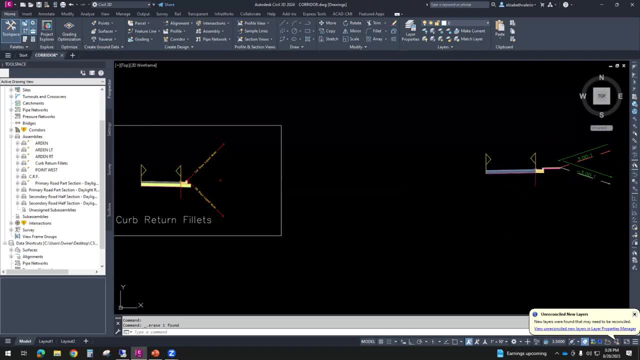 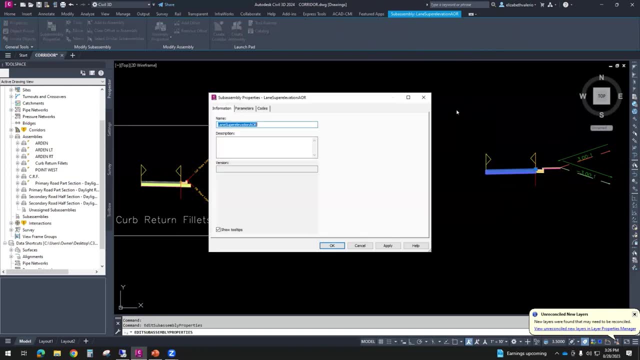 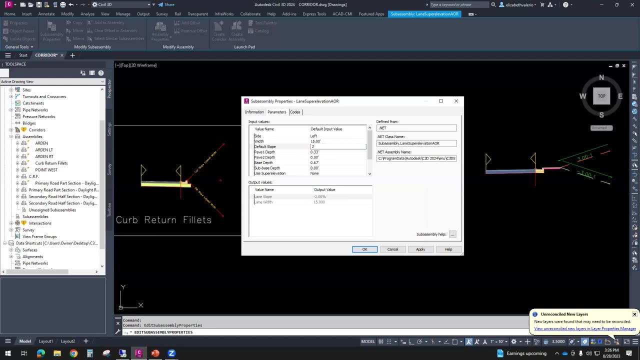 It's an easy fix. All right, All I have to do is select that sub-assembly right-click, go to Sub-Assembly Properties And on the Parameters tab, where it says negative 2%, we're going to switch it to positive 2%. 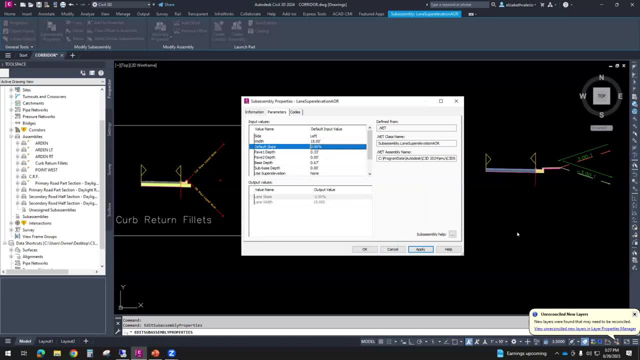 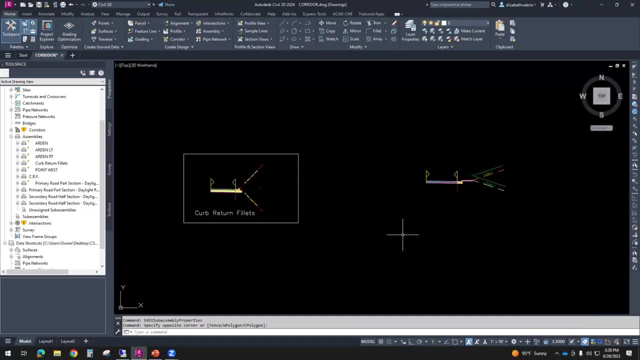 If you apply, you should see the slope changes, And that is all we need for that one. So Curb Return Fillet, We'll call that good. We have one more up here that we need to work on. So if I go up top, I'm going to copy- or, sorry, I'm going to move this. 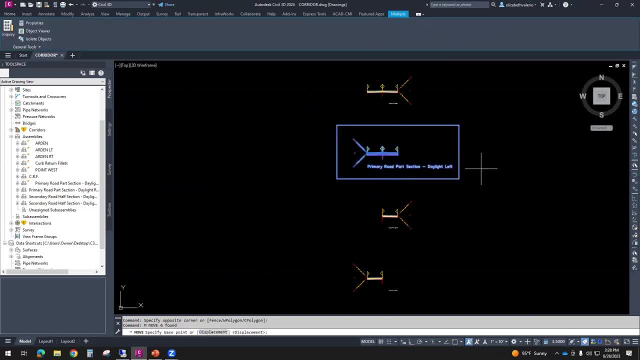 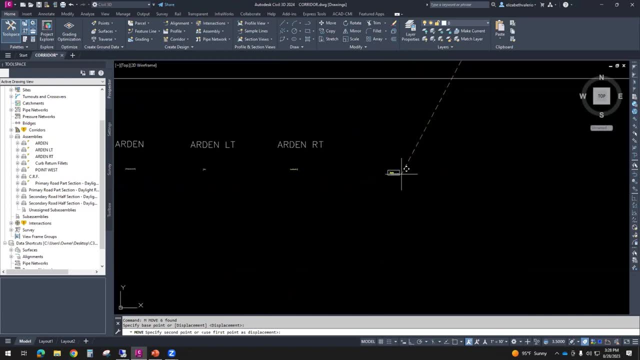 Primary Road Part Section: Daylight Left. I'm going to move that one down here And it says Primary Road, so Arden is our Primary Road. I'm going to put it in this row For Curb Return. it didn't matter. 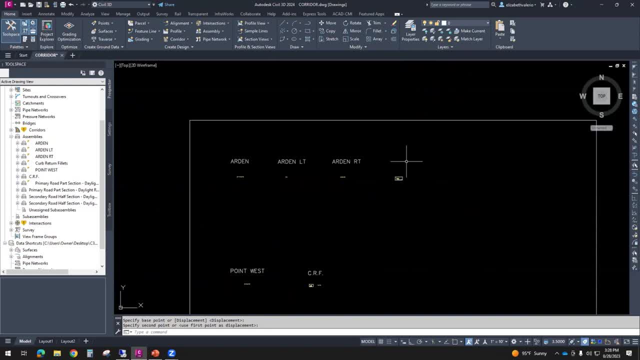 But for Primary Road. it is going to be similar to Arden. I'm going to get the original Arden copy that put it next to the one I'm working on, And we're going to give it a new name. I'm going to call it Arden Art Section. 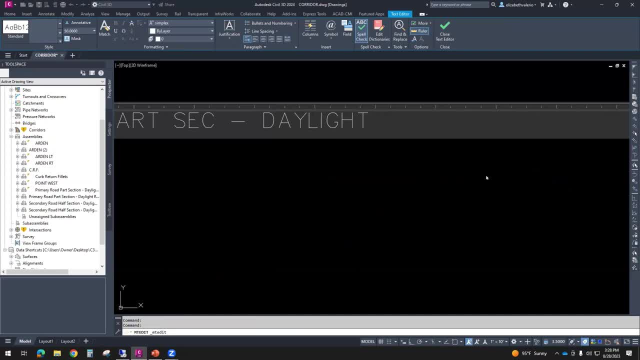 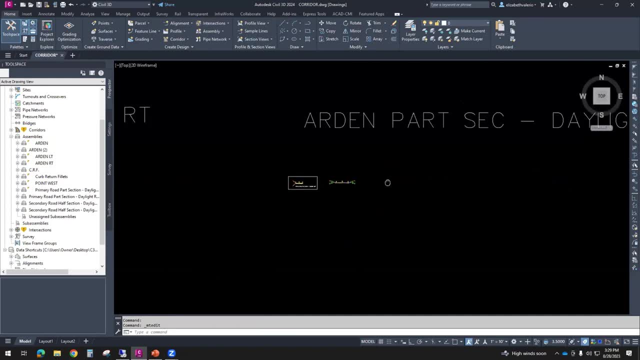 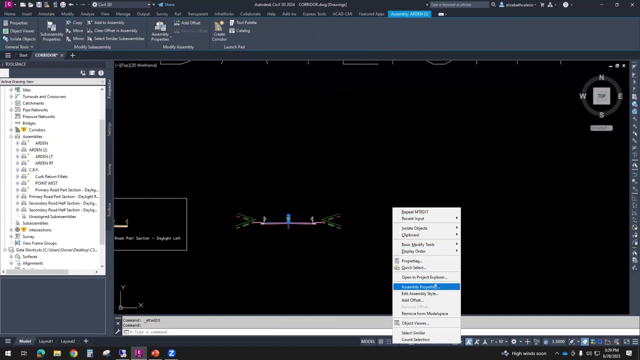 Such a long name- Daylight Left- Because it was Primary Road Part Section, Daylight Left, So Arden Part Section, Daylight Left. Once you have changed the text also, we need to rename this copy. So I'm going to grab the assembly line: right-click Assembly Properties. 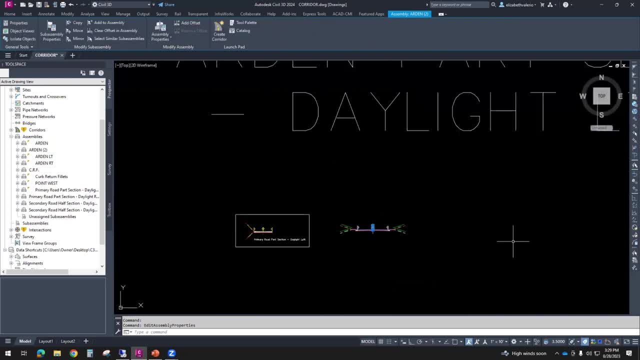 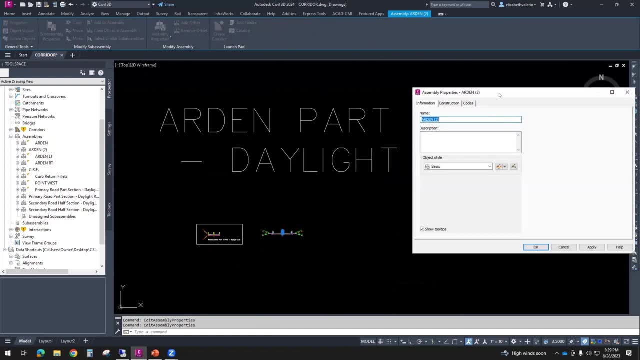 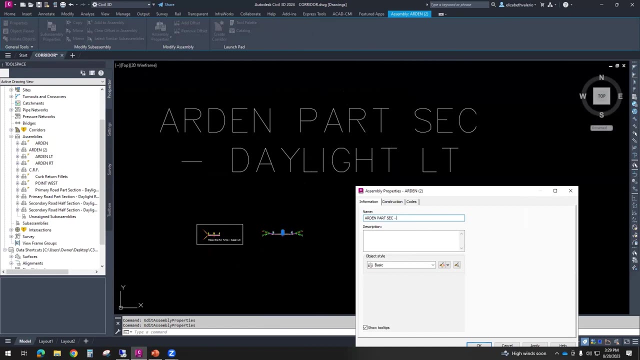 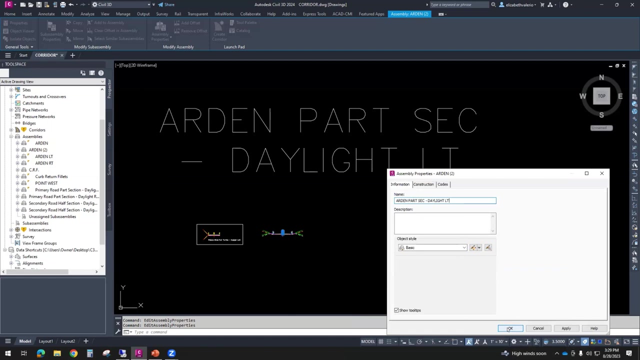 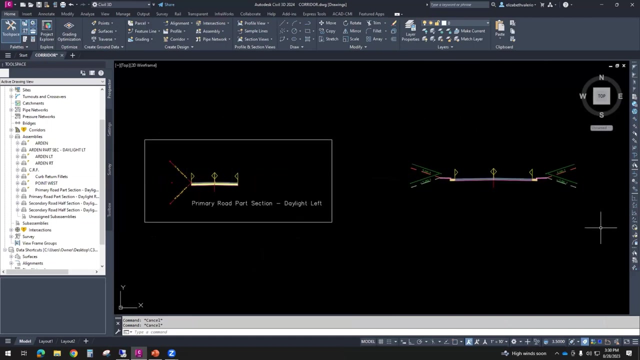 Probably should zoom out so I can see that name And then I'm going to copy that, Just changing the name. So once the name has changed, I'm going to zoom in And you're going to see what we need to do to make ours look more similar to what they have here. 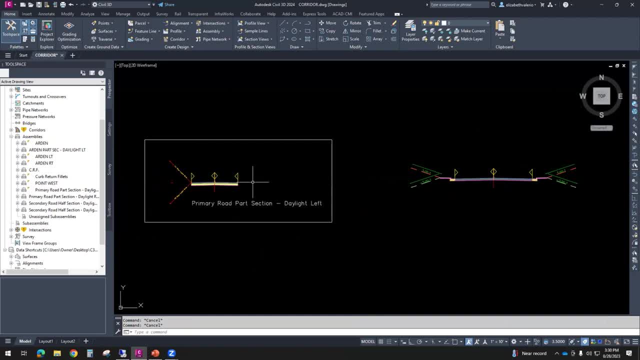 So it looks like the right half is missing. So I'm going to delete the daylight, the sidewalk and the curb and gutter. I'm going to keep the lanes and everything else All right. So now that we have created our own assemblies that we need to use in that intersection, 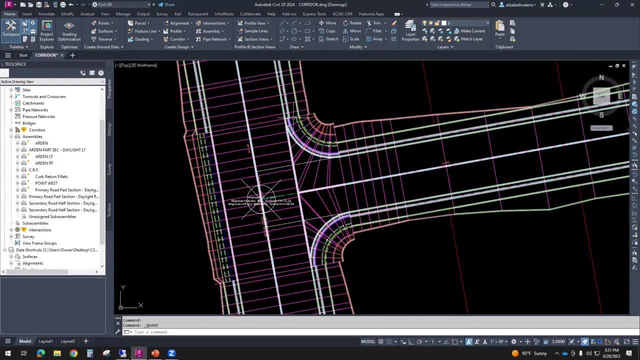 and we already saw where it looks kind of funky. right Curb returns will be replace these, And then the Daylight Left one will replace this. We can just go into Corridor Properties, So click your corridor, right-click Corridor Properties. 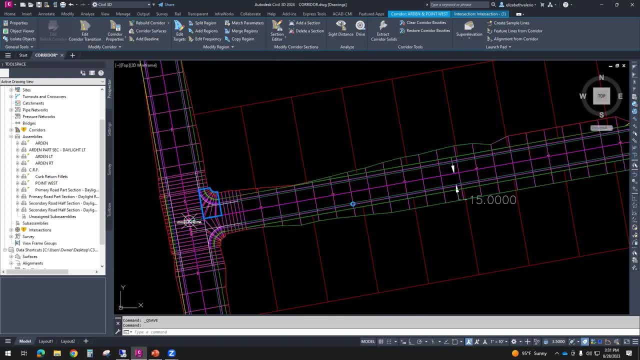 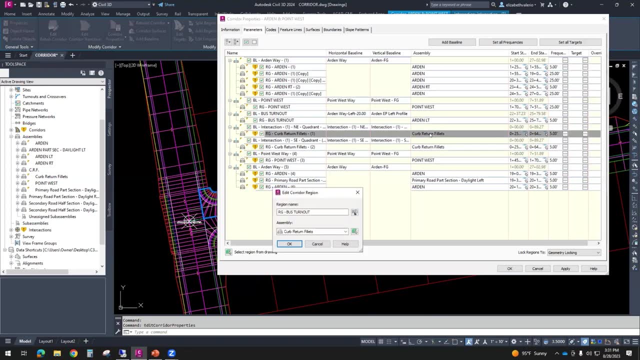 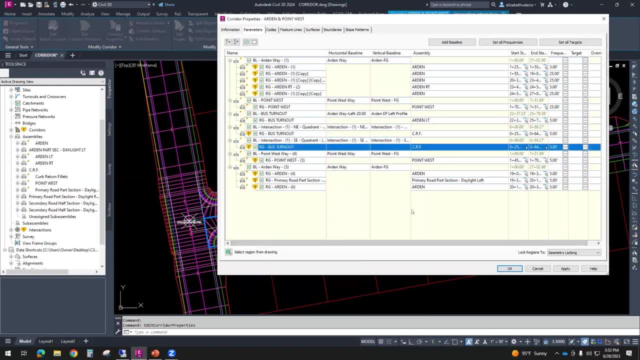 And then we're going to go back to our assemblies, And then we're going to go back to our assemblies, And then the Primary Road Part Section Daylight Left needs to be replaced with Arden Part Section Daylight Left. So once we're using all of our own assemblies, we can click OK, rebuild. 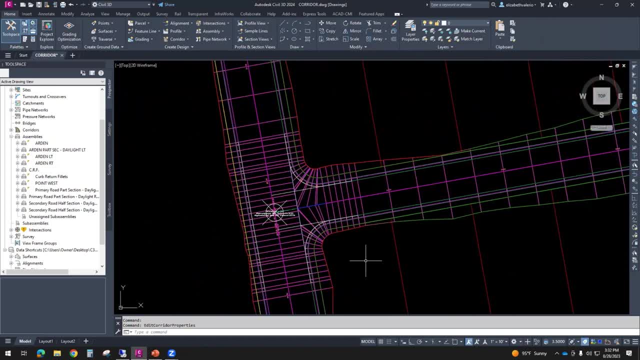 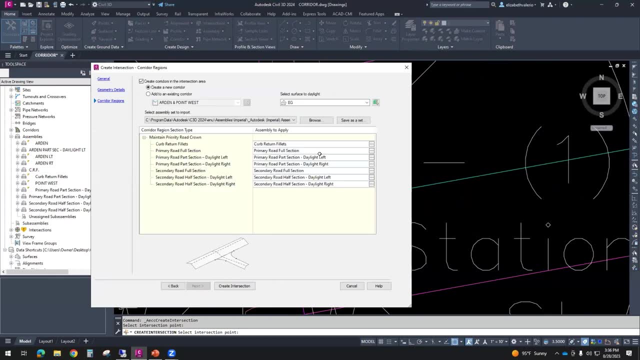 And it should look nice and smooth, matching up with our design. It should look nice and smooth, matching up with our design, our design. All right, so on this page, these are the default ones that come with the program. If you have your own, like someone said, they have their own company assemblies- you can. 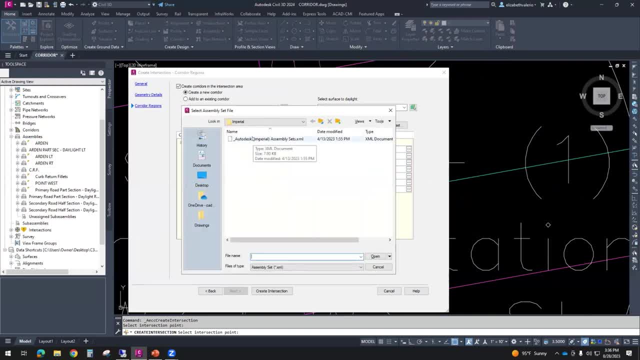 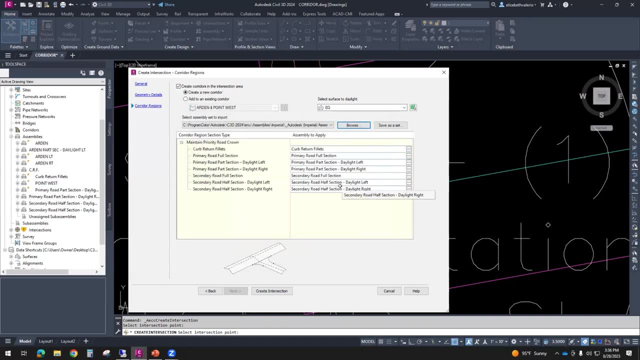 browse and then select your saved list of assemblies And then that can populate this automatically. Like for right, now we are all starting from scratch, right. But now that I've done this I can say, okay, this is actually CRF And this is actually Arden, And this is Arden. 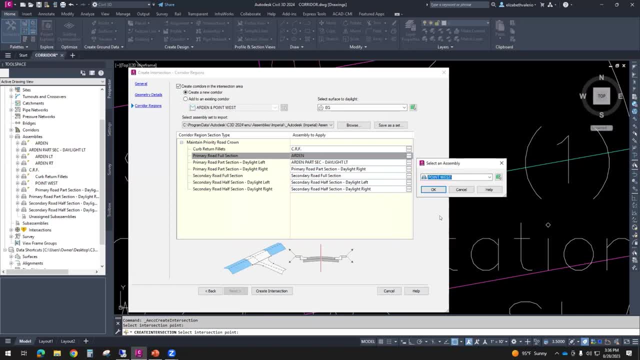 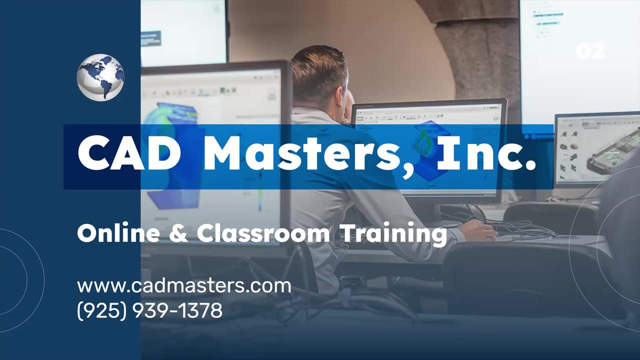 And that is West right, What I can do here. once I've assigned everything that I need, I can save it as a Set And that creates this XML file. Admasters offers online and classroom training for a variety of Autodesk software. 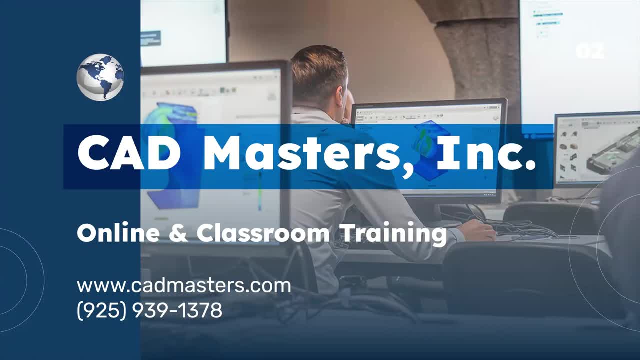 For more information, go to wwwcadmasterscom or give us a call at 925-939-1378..